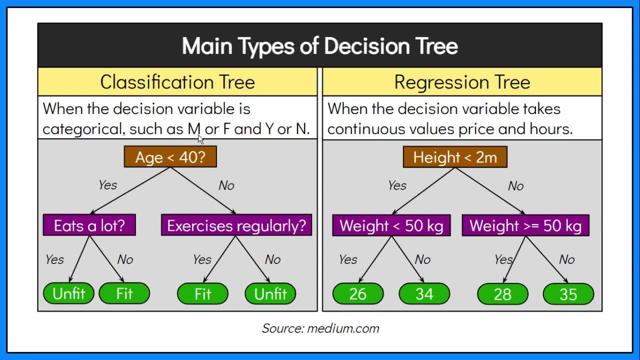 tree. When the decision variable is categorical, such as fit or unfit, yes or no, true or false, male or female, it forms a classification tree. On the other hand, it is called a regression tree when its outcome variable takes continuous values, Typically real numbers such as price. 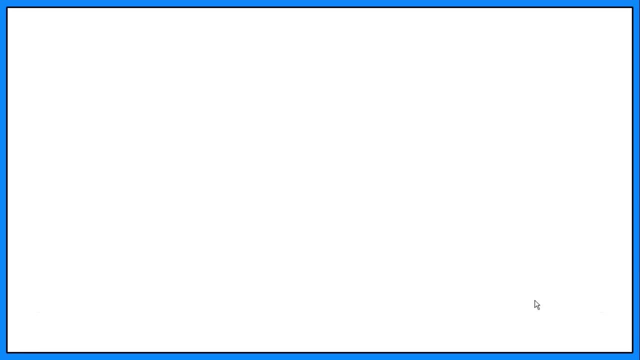 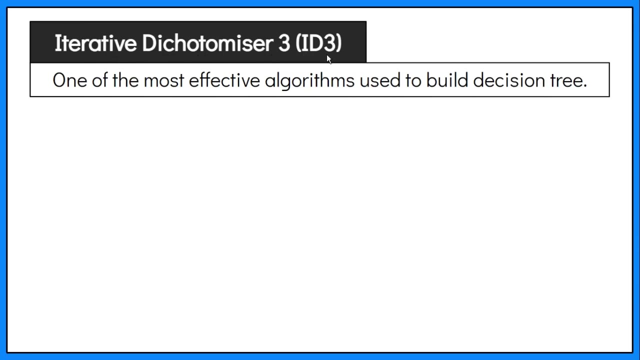 hours, sales and profit. One of the most effective algorithms used to build decision trees is Iterative Dichotomizer 3 or ID3. It uses two measures to generate a decision tree for a given dataset. First, entropy: It is the measure of impurity, disorder or uncertainty in a bunch of sample. 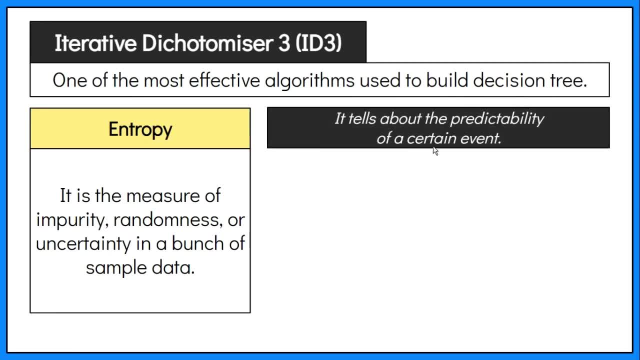 data. It tells about the predictability of a certain event. It controls how a decision tree decides to split the data. To illustrate this, imagine you are to pick a fruit in a basket that only contains apples. It can be predicted perfectly, Since we know beforehand that it will always be an apple. In this case, entropy is zero. 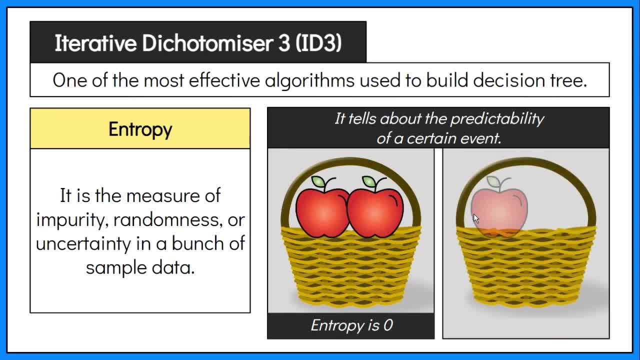 since the event has no randomness. On the other hand, if a basket contains two kinds of fruits- one apple and one orange- the entropy in this case is the highest possible, since any of the two fruits can be randomly selected. Take note that lower entropy values imply less uncertainty, while higher values imply. 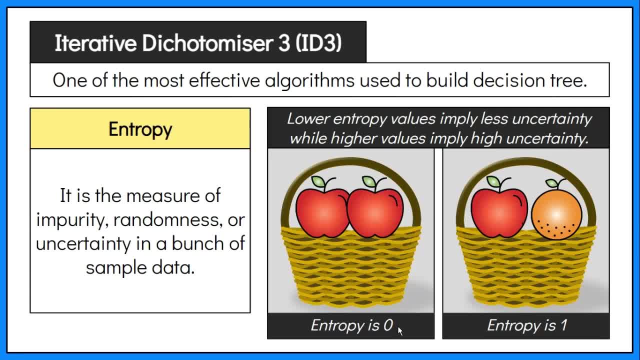 high uncertainty. entropy values range from zero to two values of uncertainty. Transmitted values are quite random. There is no set of logic for the higher values and that means that I don't know if I could get the answer to that. So more or less I will figure out. 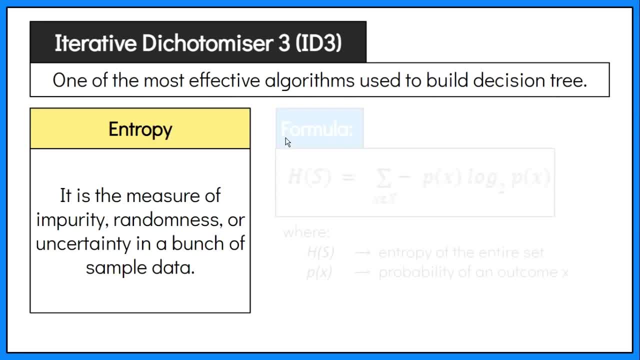 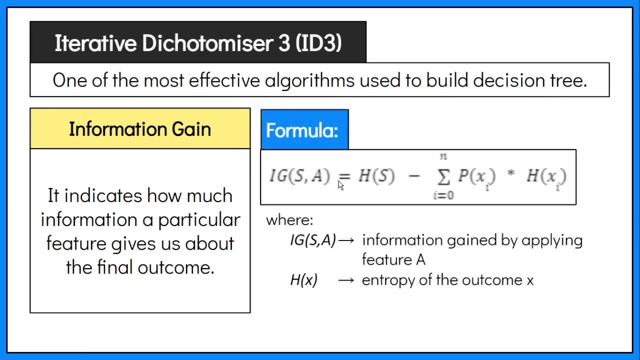 to one only. This is the formula of entropy. Second information gain: It indicates how much information a particular feature gives us about the final outcome. It is important because it is used to choose the feature that best splits the data at each node of a decision tree. This is the 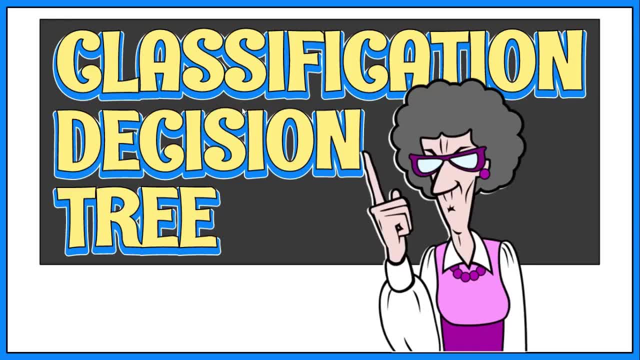 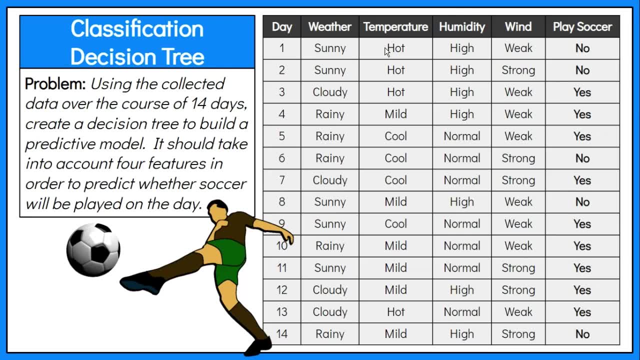 formula To understand these concepts better. let's have an example. Consider. these data have been collected in the course of 14 days. The following features have been observed and recorded: Weather, temperature, humidity and wind. The target variable or outcome is whether soccer was played or not on that day. Now, using 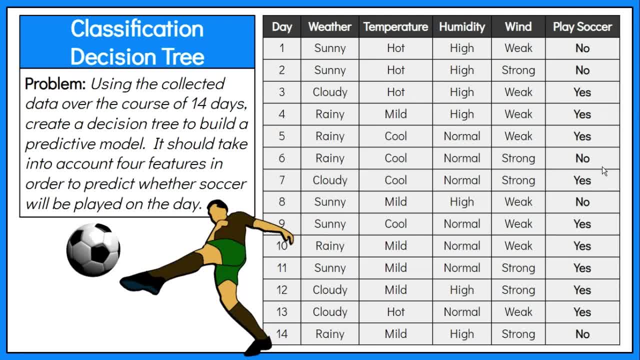 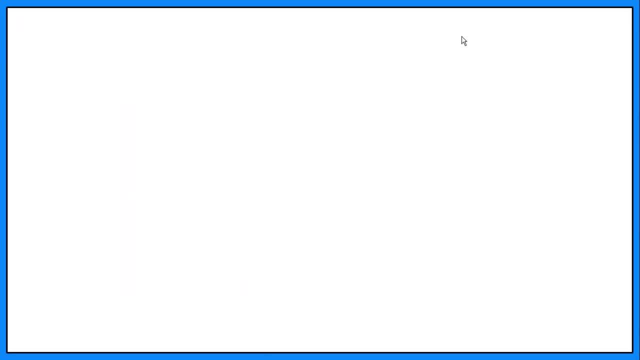 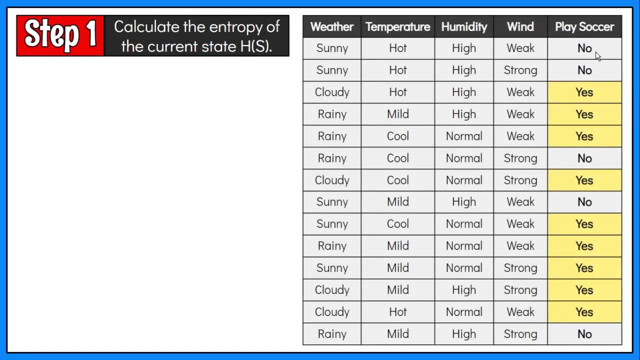 the gathered data, let's create a decision tree to build a predictive model that will identify whether soccer will be played, based on the specified four features. Step 1. Calculate the entropy of the current state In the target variable, which is play soccer. we found two outcomes, namely yes and no. 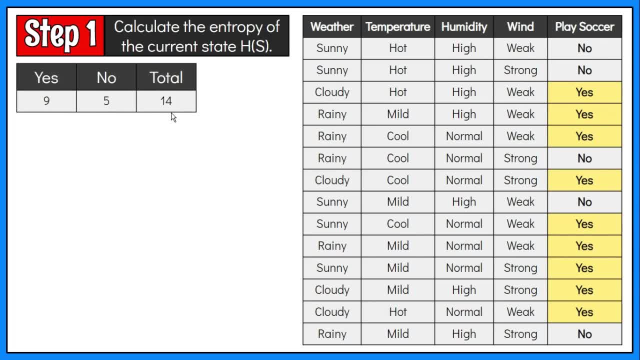 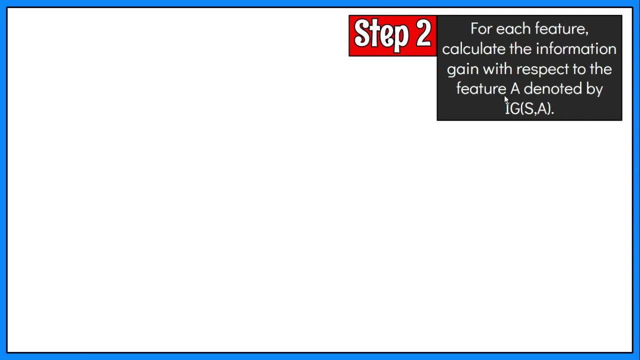 There are nine samples with yes, while five with no. Using the formula, we got the entropy of the entire data set, and that is 0.940.. Step 2. For each feature, calculate the information gain with respect to the set feature. Let's start with a feature wind. Based on the sample data, it takes two. 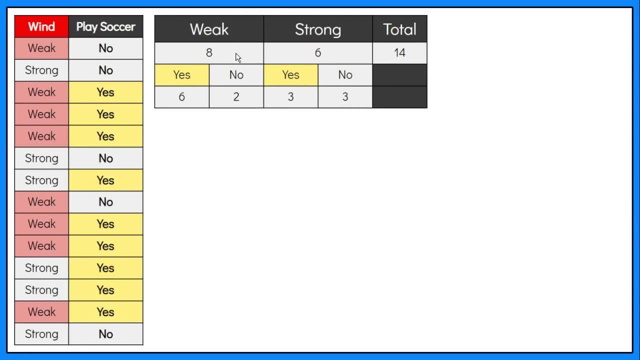 possible values. Weak and strong. There are eight instances of weak and six for strong. Out of the eight weak examples, six of them were yes, for play soccer, and two of them were no. And out of the six strong examples, three of them were yes and three of them were 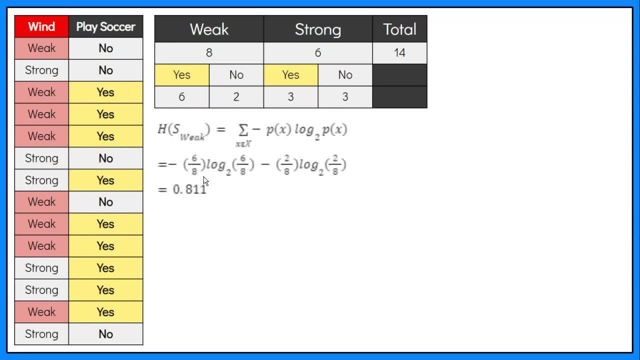 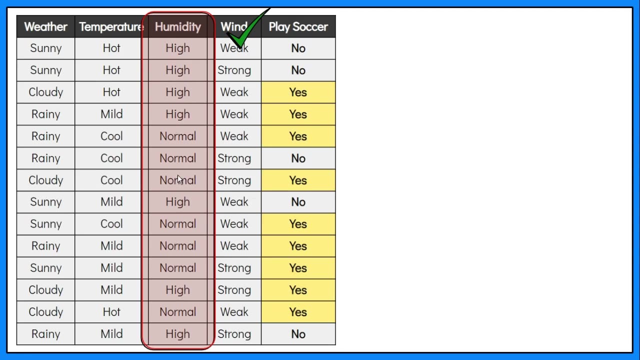 no. After computing, the entropy for weak is 0.811 and the entropy for strong is 1.. Using the formula for information gain, we got 0.048.. Next let's compute the humidity feature Based on the sample data. it takes two possible. 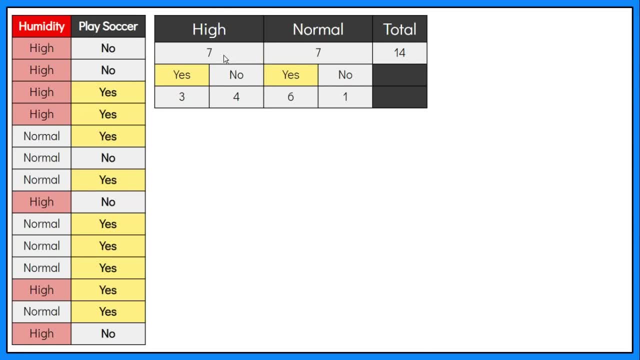 values, high and normal. There are seven instances of high and seven for normal. Out of the seven high examples, three of them were yes and four of them were no, while out of the seven normal examples, six of them were yes And one of them was no. 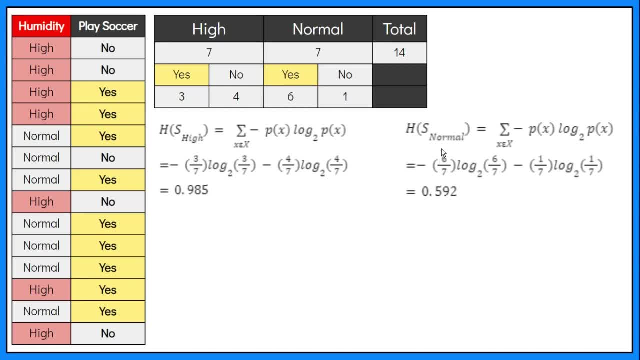 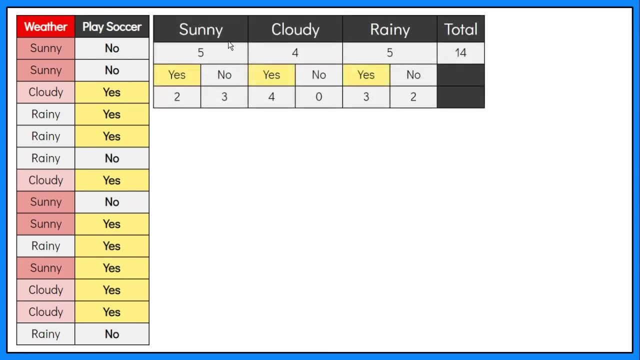 After computing, the entropy for high is 0.. lie five and the entropy for normal is 0.98.. 0.592.. Using the formula for information gain, we got 0.152.. Let's move to the next feature, which is weather Based on the sample data. it takes three possible. 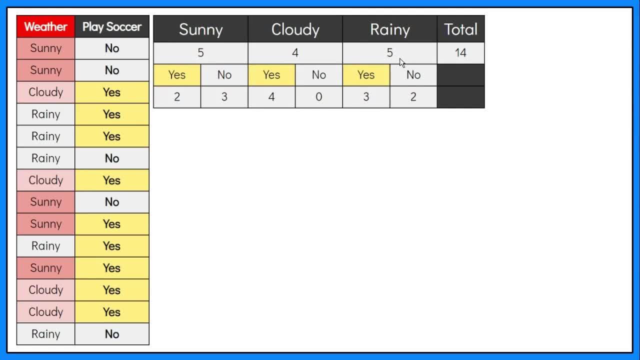 values: sunny, cloudy and rainy. There are five instances of sunny, four for cloudy and five for rainy. Out of the five sunny examples, two of them were yes and three of them were no. Out of the four cloudy examples, four of them were yes and none of them was no. Out of the five examples, 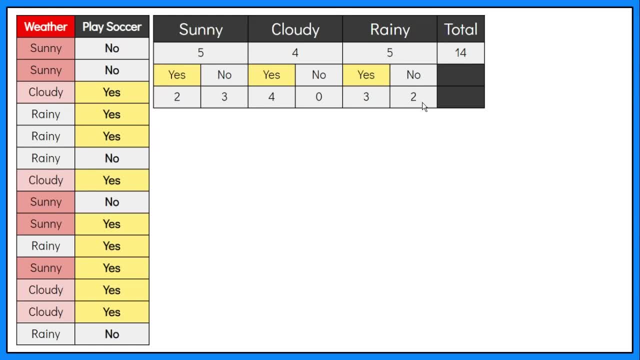 three of them were yes and two of them were no. After computing, the entropy for sunny is 0.971, zero for cloudy, since all the instances go to yes outcome only, and 0.971 for rainy. Using the formula for information gain, we got 0.246.. 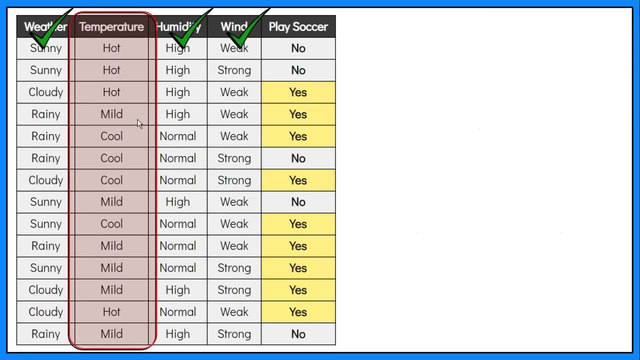 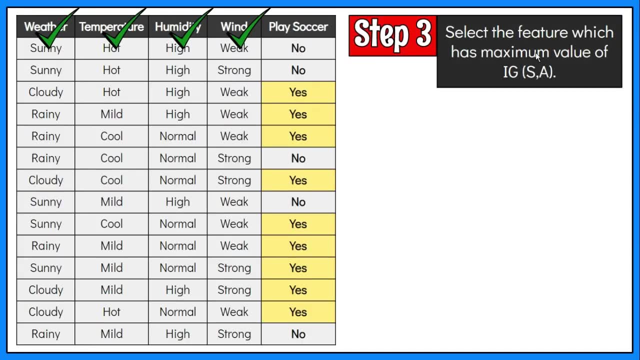 Now let's move on to the next feature, which is weather. Based on the sample data, it takes three possible values: hot, mild and cool. Step three: select the feature which has maximum value of information gain Based on our computation. in step two, the weather feature has: 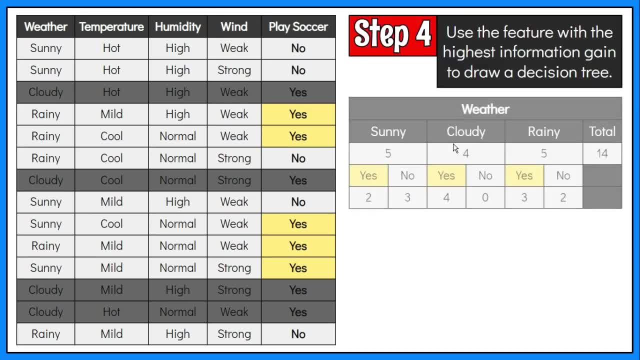 the highest value, The weather feature becomes the root node. There are three branches. since there are three possible values for the weather feature, namely sunny, cloudy and rainy, Upon checking it shows that the yes has four and no has zero, We can now put a leaf node in the 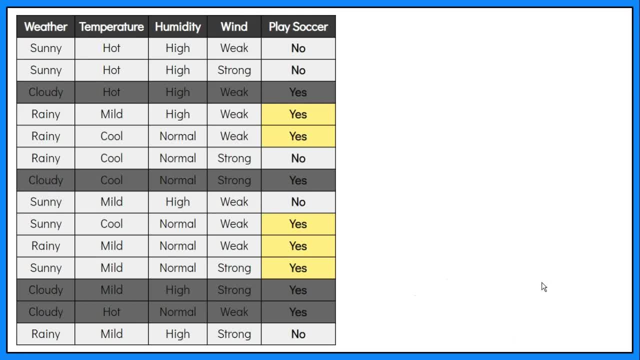 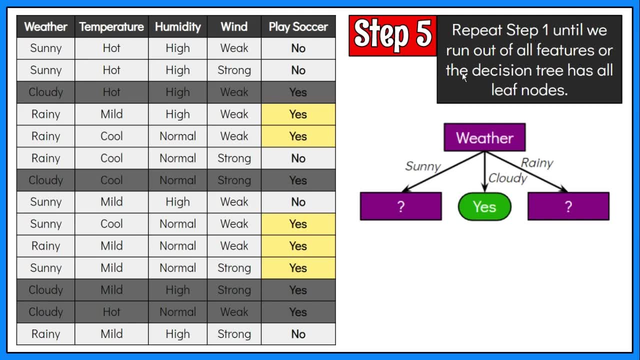 cloudy branch, Its value is yes. For the sunny and rainy branches, we will compute entropy and information, gain Step five, repeat step one until we run out of all features or the decision tree has all leaf nodes. This will be done to find out what feature will be connected to the branch. 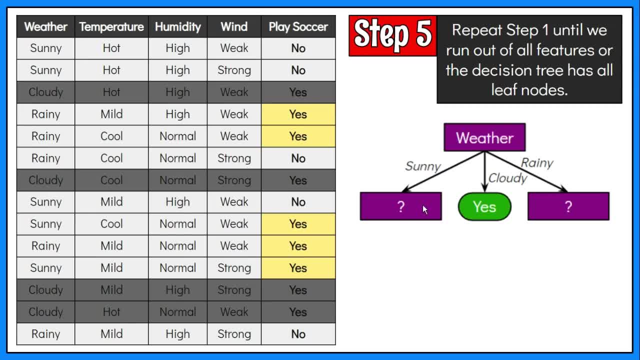 from the root node, Let's identify what feature can be put in the leaf node. The leaf node will be the decision node that can be connected to the sunny branch. then for the rainy branch We'll remove weather from the set of features. for the next iteration Let's start with step number one. 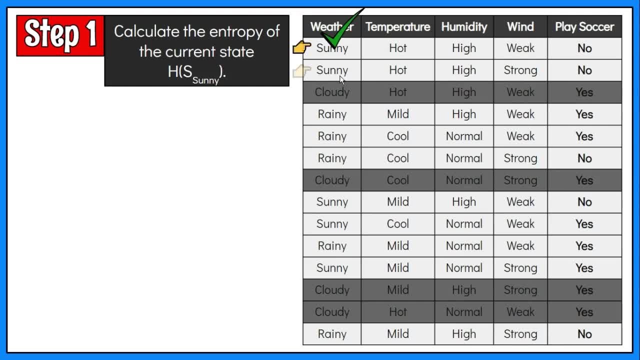 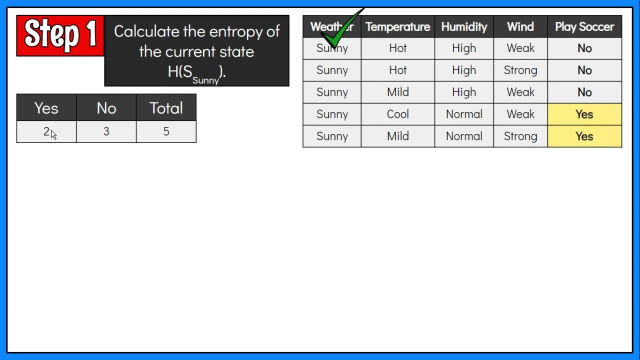 Calculate the entropy for the current state At this point. let's find the sunny examples in the weather feature For this calculation. the total outcome that is taken into consideration is five. We found two yes and three no values. Using the formula, we get the entropy of the entire set. 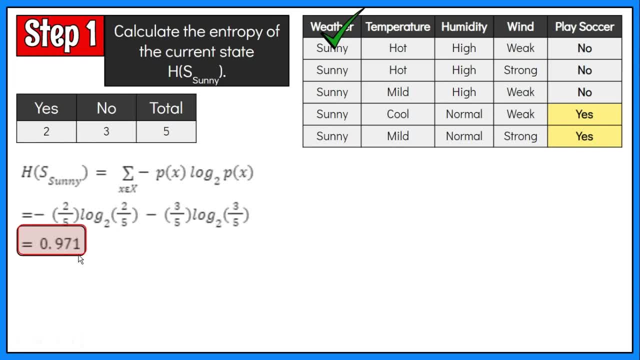 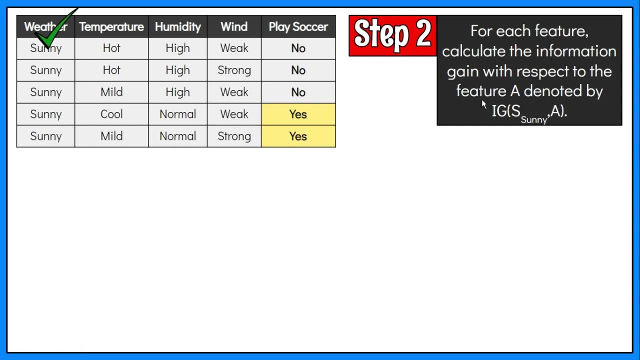 for the sunny element of weather feature, and that is 0.971.. Step two: for each feature, calculate the information gain with respect to the set feature. Let's start again with the feature wind. There are three instances of weak and two for strong. After computing the entropy for weak, 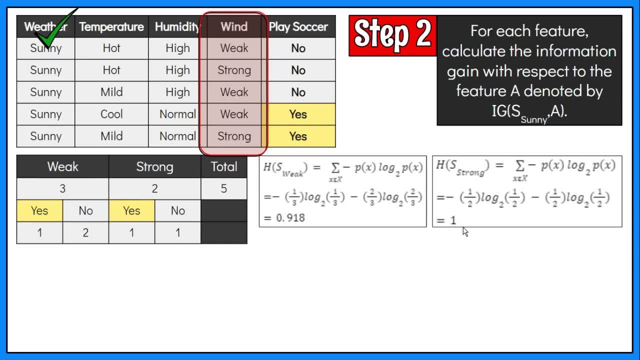 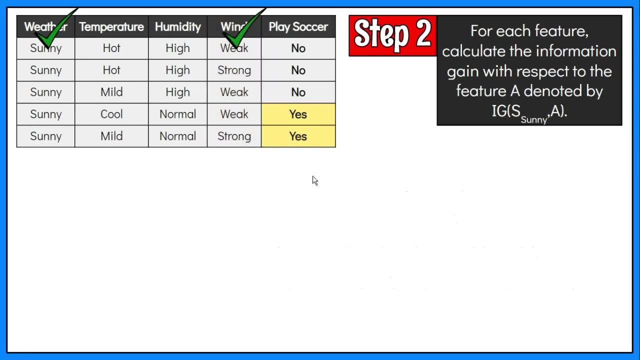 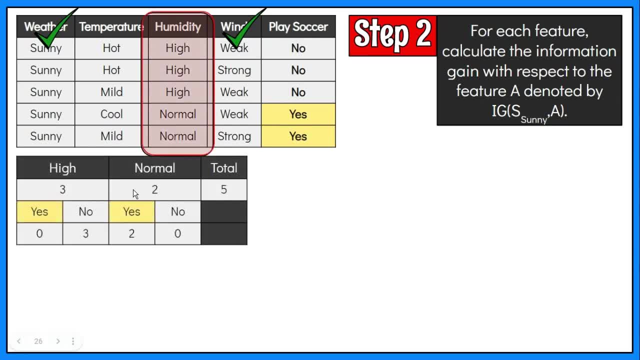 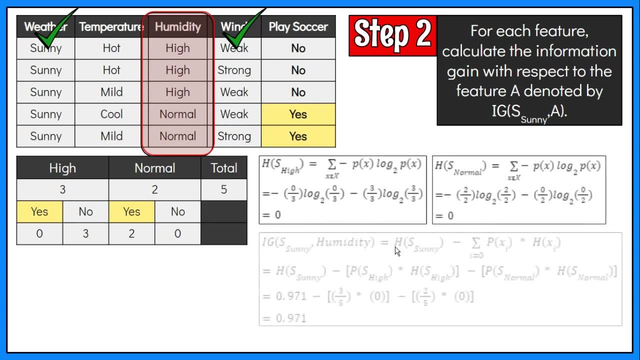 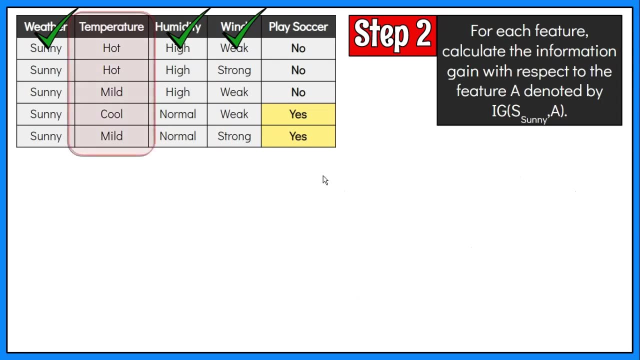 There are three instances of high and two for normal. After computing, the entropy for both high and normal is zero. Using the formula for information gain, we got 0.971.. This time let's compute the temperature feature. There are two instances of hot. 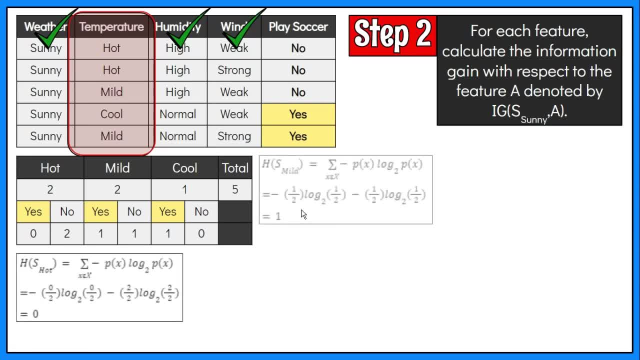 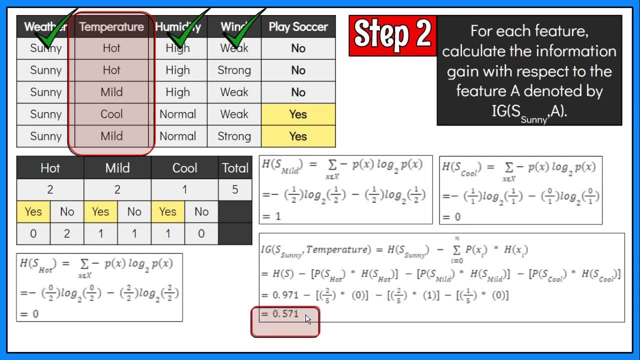 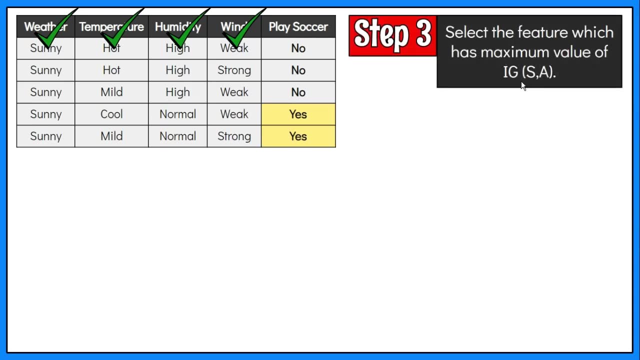 two for mild and one for cool. After computing, the entropy for hot is zero, one for mild and zero for cool. Using the formula for information gain, we got 0.571.. Step three: select the feature which has maximum value of information gain. 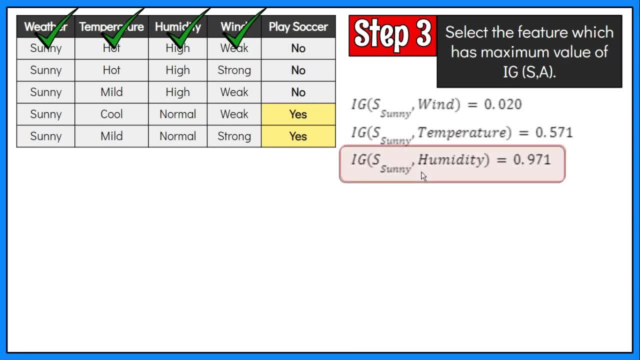 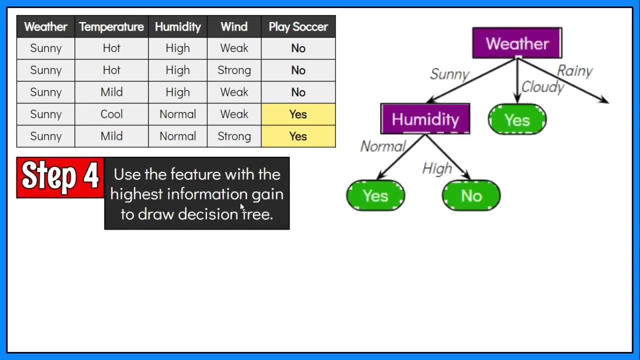 These are all the values we have computed. for information gain, The humidity feature has the highest value. Step four: using the feature with the highest information gain, draw a decision tree Now that we know humidity has the highest information gain for sunny branch computation. 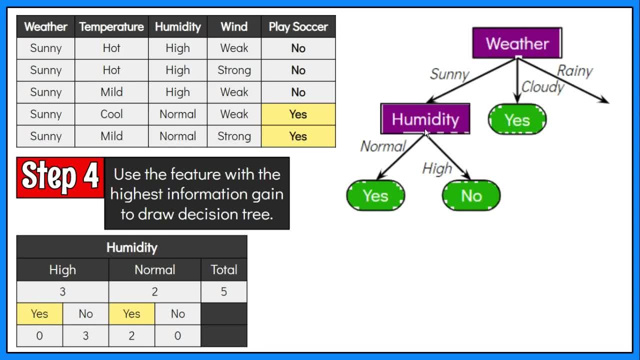 the humidity feature becomes the decision node, We will connect humidity to the branch from the weather root node. There are two branches from humidity, since there are two possible values: normal and high. Upon checking the examples, it shows the node has three. Therefore, we can now put a leaf node in the high branch. 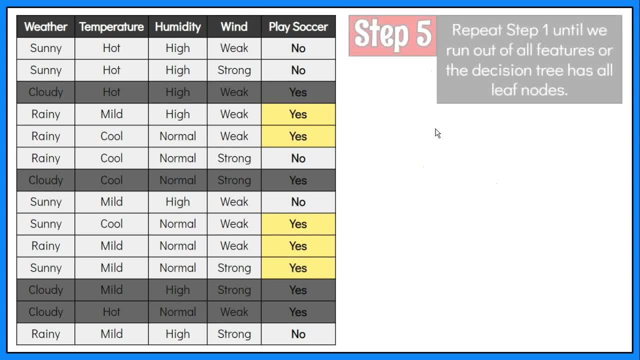 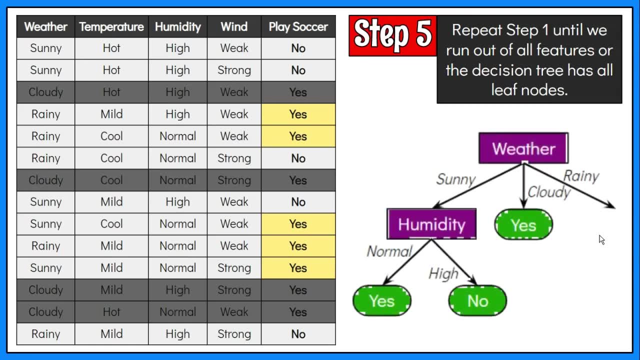 The value is no. Step five: repeat step one until we run out of all features or the decision tree has all leaf nodes. Step six: we can now put a leaf node in the high branch. The value is no. Looking at our decision tree, we still have to find the decision node for the rainy branch. 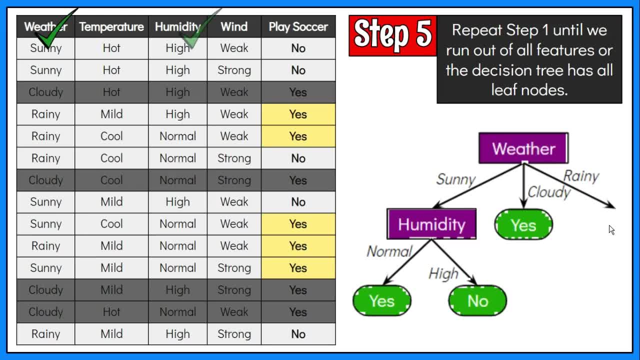 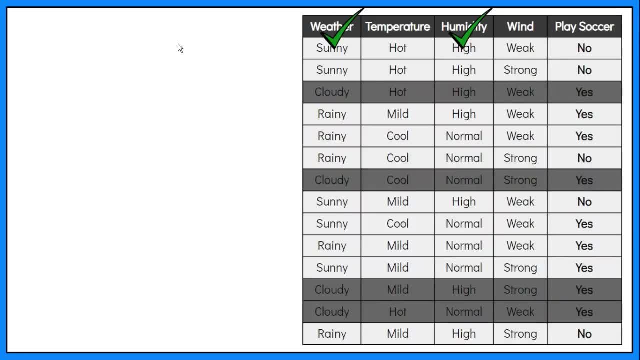 so we will do the same procedure. Aside from weather, we will also remove humidity from the set of features. for the other branches- computation- We'll go back to step one: Calculate the entropy of the current state. Let's find the rainy samples in the weather feature. 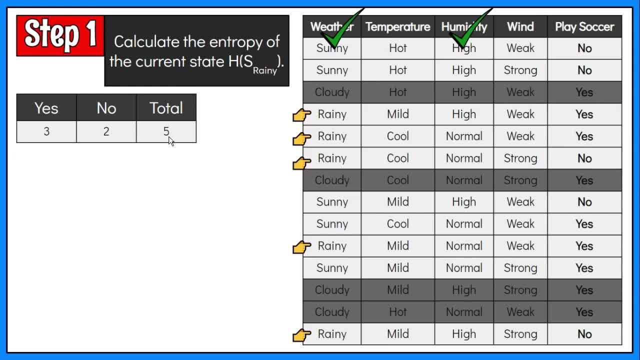 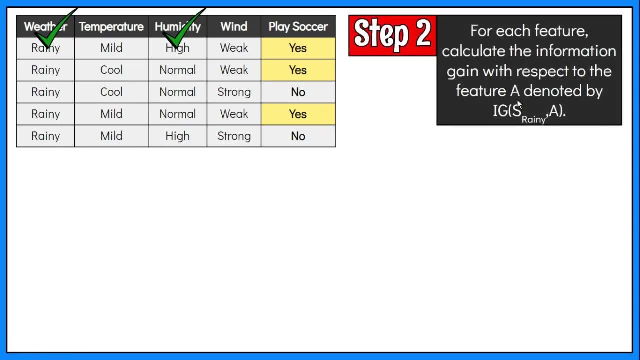 For this calculation, the total outcome that is taken into consideration is five. We found three values and two no values. The computed entropy is 0.971.. Step two: for each feature, calculate the information gain with respect to that feature.